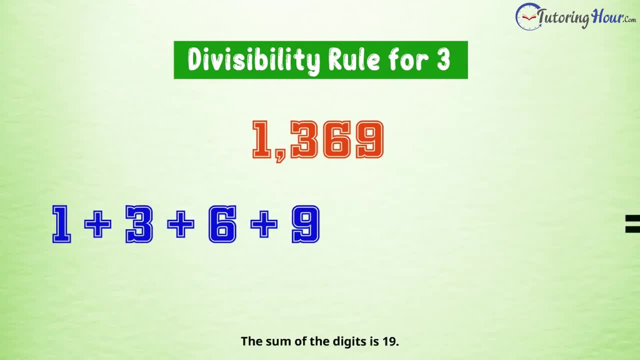 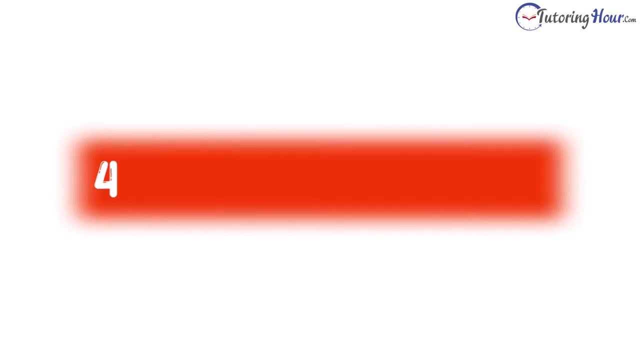 on another number. The sum of the digits is 19.. 19 is not divisible by 3.. It is quite clear that 1369 is also not divisible by 3.. Now, that was a pretty simple rule. Moving on, we'll try the divisibility rule for 4 on the number 778.. 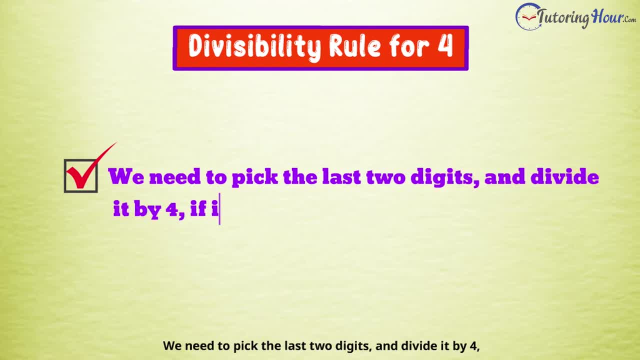 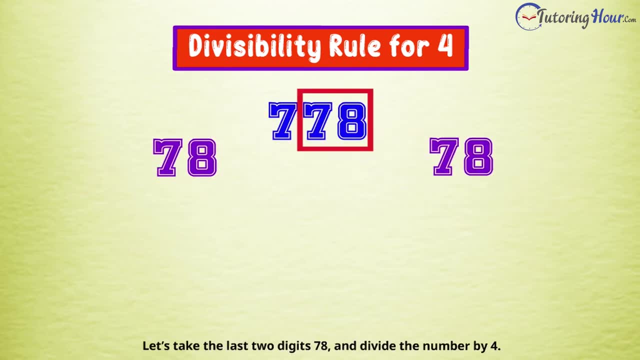 We need to pick the last two digits and divide it by 4.. If it leaves no remainder, the number is divisible by 4.. Let's take the last two digits- 78, and divide it by 4.. We are left with 2 as the remainder. 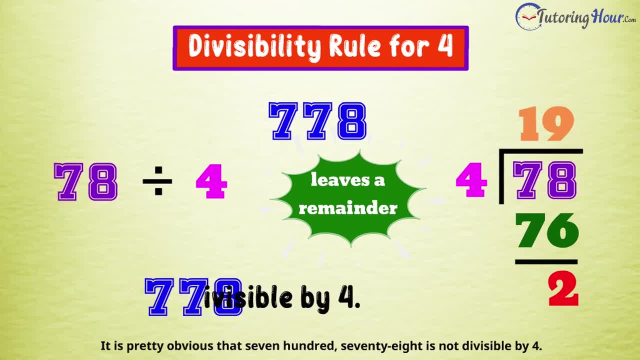 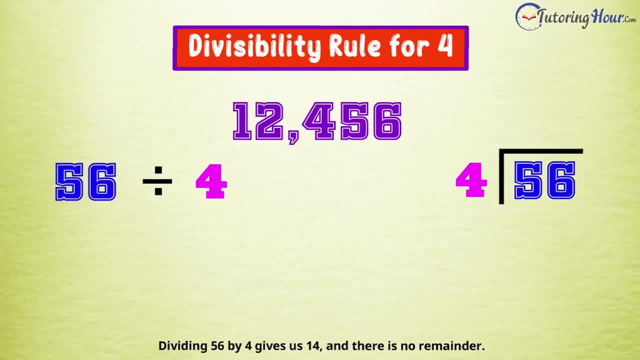 It is pretty obvious that 778 is not divisible by 4.. Now we'll check if our next number is divisible by 4.. Dividing 56 by 4 gives us 14, and there is no remainder. This shows the number is divisible by 4.. 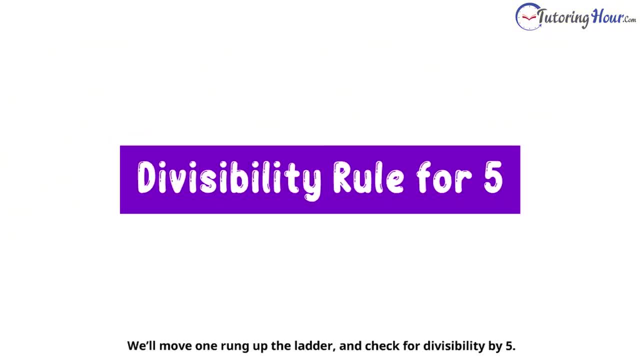 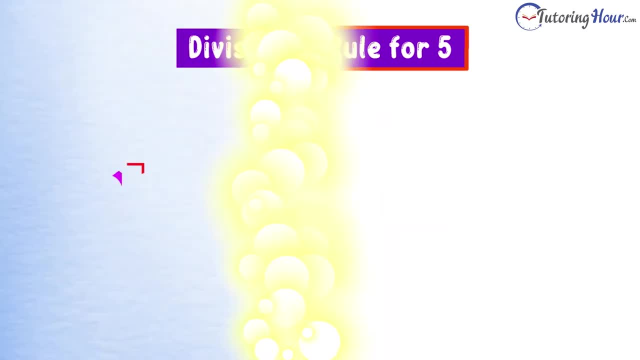 OK, We'll move one rung up the ladder and check the divisibility by 5.. Is the number 154 divisible by 5?? The rule states a number is divisible by 5 if it has 0 or 5 in its ones place. 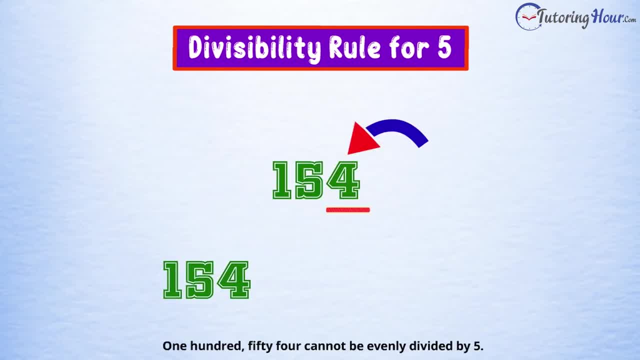 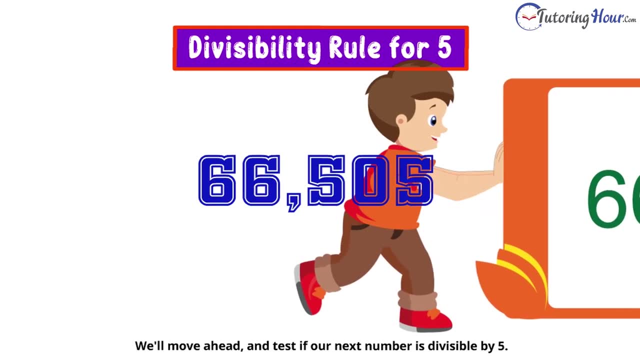 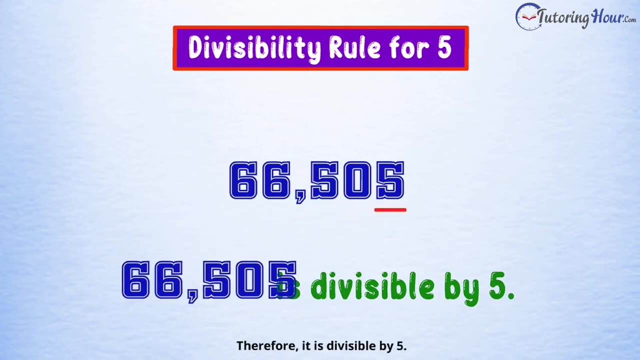 The number 4 in the ones place hints that 154 cannot be evenly divided by 5.. We'll move ahead and test if our next number is divisible by 5.. Keeping in step with the rule of 5,, this number ends in 5, therefore divisible by 5.. 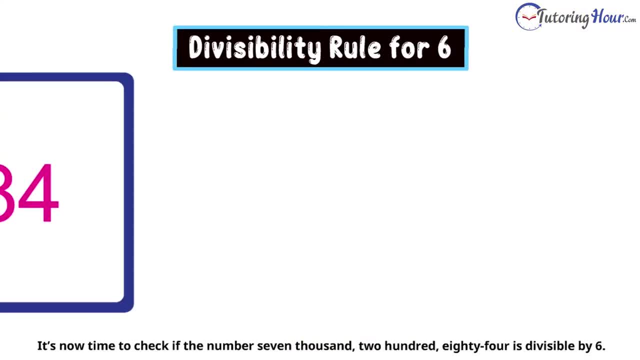 Pretty simple stuff. It's now time to check if the number 7284 is divisible by 6.. The rule is: if a number is divisible by 2 and 3, then it is divisible by 6 as well. Let's recall the divisibility rule for 2,. 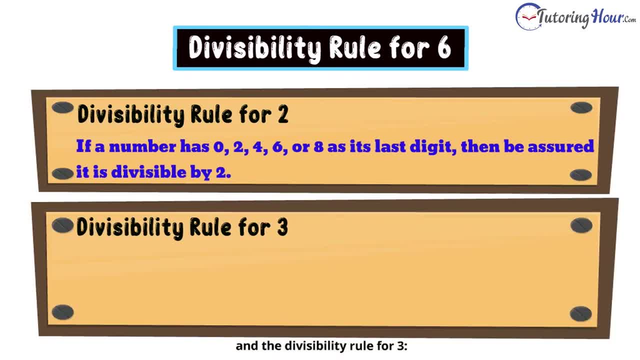 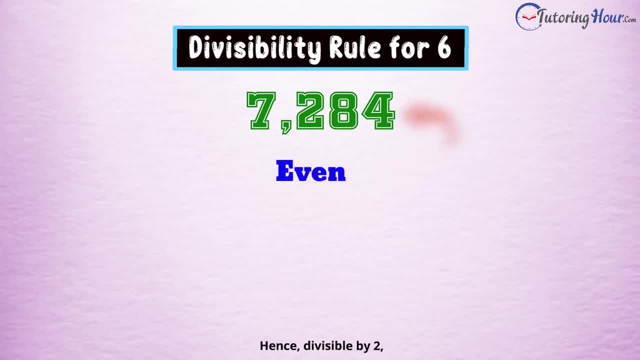 which is, and the divisibility rule of 3, which is, Without doing too much calculation, we know it is even hence divisible by 2.. Hold on, we're not done yet. We need to check if it is divisible by 3 as well. 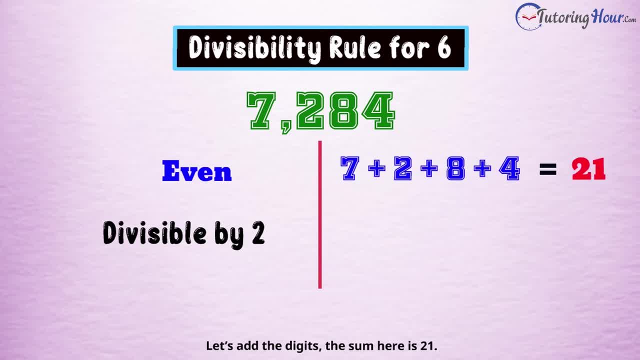 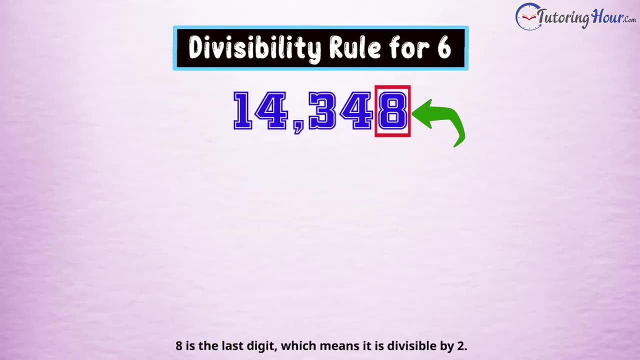 Let's add the digits. The sum here is 21.. It is pretty clear: 21 is divisible by 3.. Since the number satisfies both the conditions, it is divisible by 6.. We'll test one more number. 8 is the last digit. 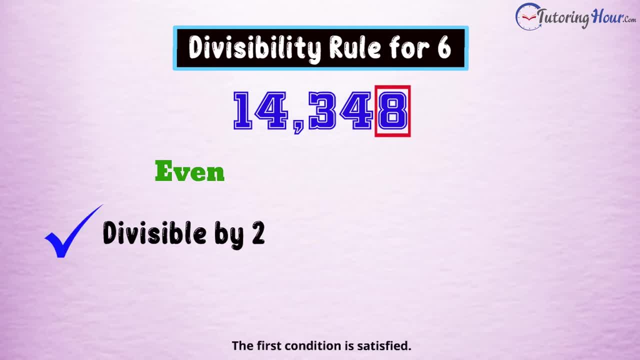 Which means it is divisible by 2.. The first condition is satisfied. Let's see if it is divisible by 3. Adding all the digits, we get 20.. 20 is not divisible by 3. It doesn't meet the second requirement. 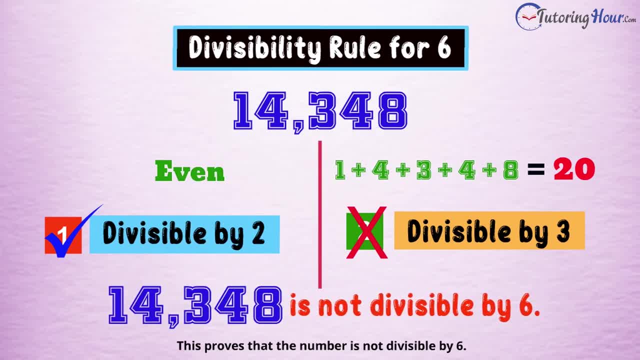 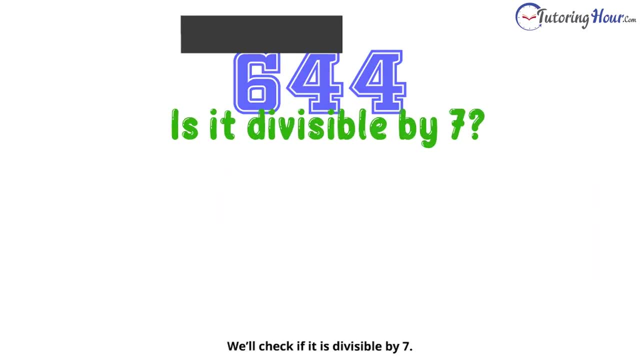 This proves that the number is not divisible by 6.. That leads us to our next number, which is 644.. We'll check if it is divisible by 7.. We need to double the last digit and subtract it from the number formed by the other digits. 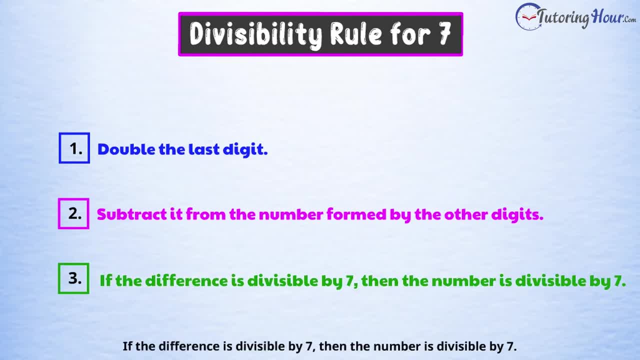 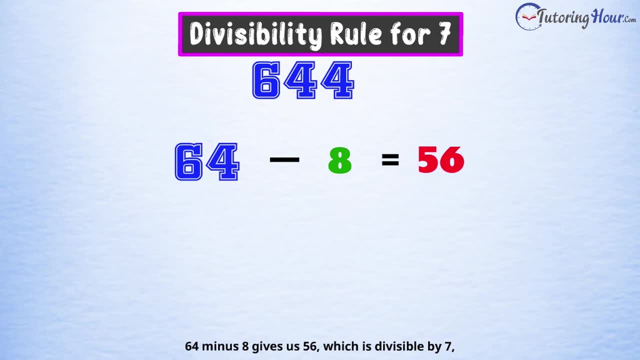 If the difference is divisible by 7,, then the number is divisible by 7.. Doubling the last digit, we have 8.. 64 minus 8 gives us 56,, which is divisible by 7.. Therefore, we can conclude that the number is divisible by 7.. 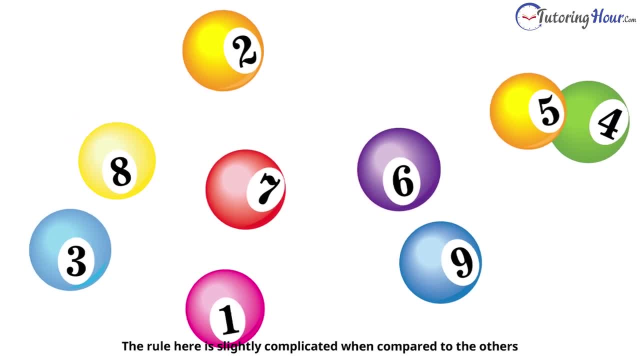 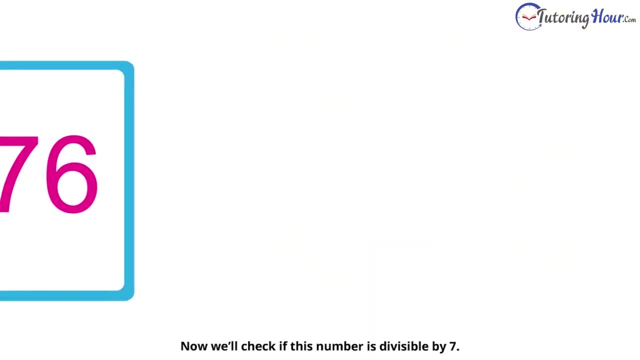 The rule here is slightly complicated when compared to the others. Nonetheless, with a little practice you can surely outwit your peers. Now we'll check if this number is divisible by 7.. Doubling the last digit, 6,, we get 12.. 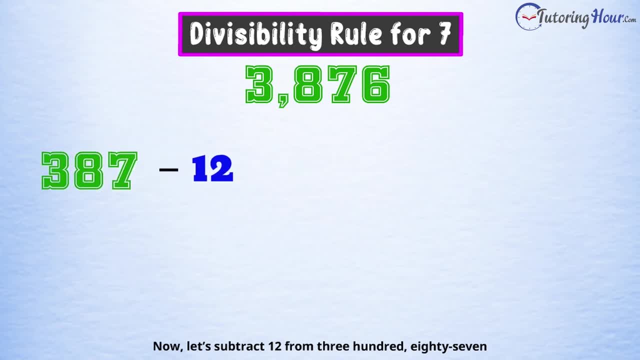 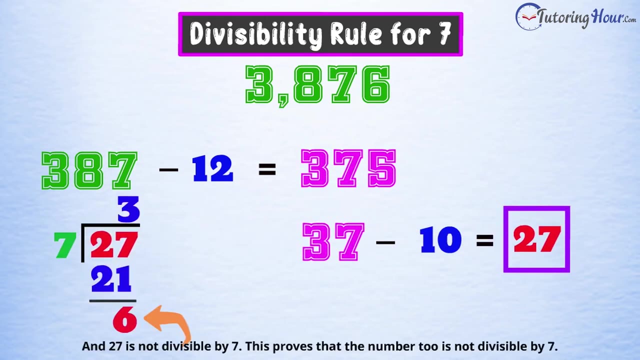 Now let's subtract 12 from 387, which leaves us with 375.. We'll repeat the process. Doubling the last digit, 5, gives us 10.. 37 minus 10 is 27,, and 27 is not divisible by 7.. 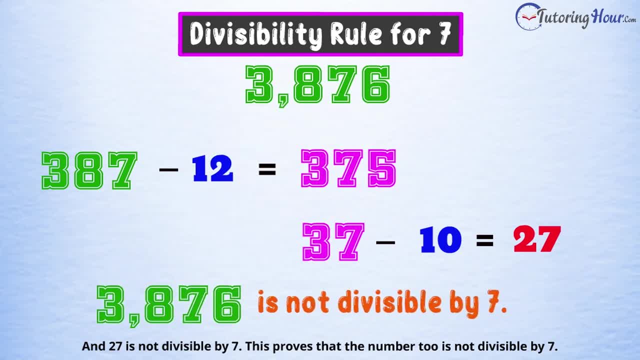 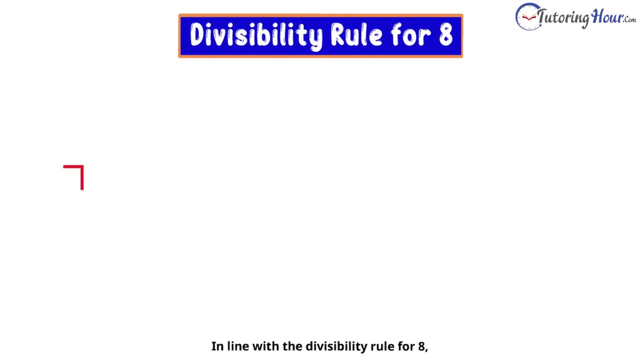 This proves that the number 2 is not divisible by 7.. We'll test if this number is divisible by 8.. In line with the divisibility rule for 8, that says, if the last three digits are divisible by 8,, then the number is divisible by 8.. 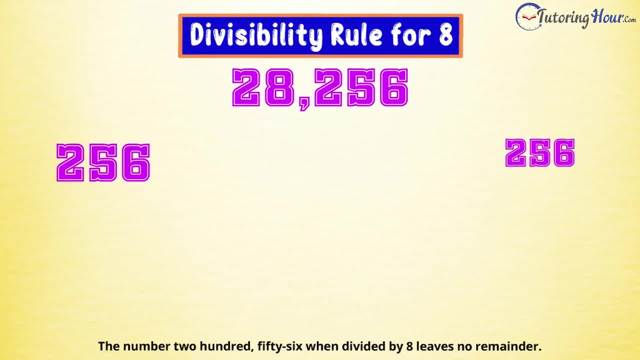 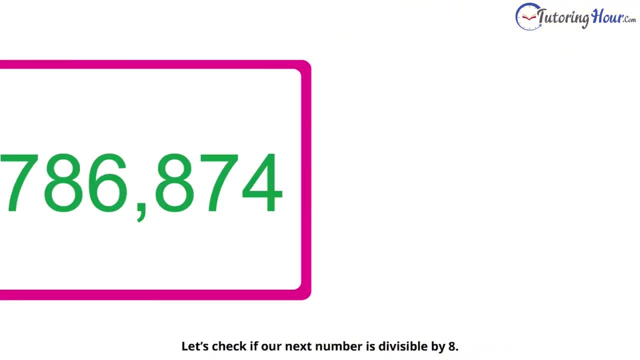 The number 256, when divided by 8, leaves no remainder indicating the entire number is divisible by 8.. Let's check if our next number is divisible by 8.. 874, when divided by 8, leaves a remainder 2,. 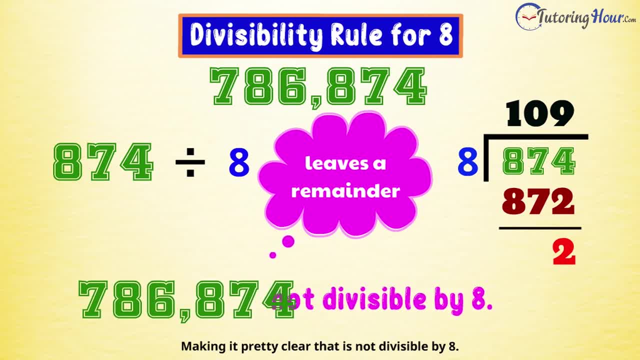 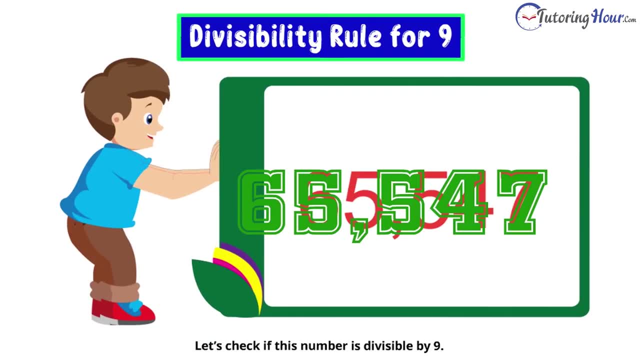 making it pretty clear that it is not divisible by 8.. That's a pretty cool rule. Coming up next is the test for divisibility by 9.. Let's check if this number is divisible by 9.. The rule for 9 is similar to the rule for divisibility by 3.. 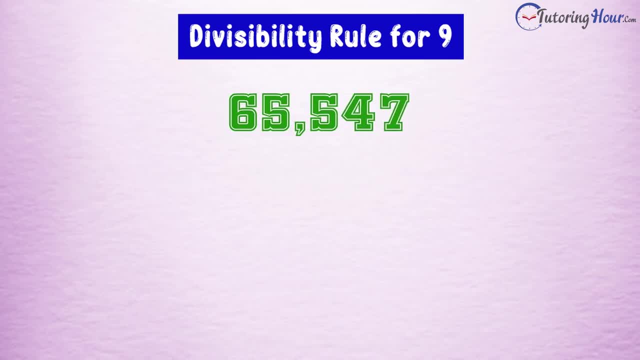 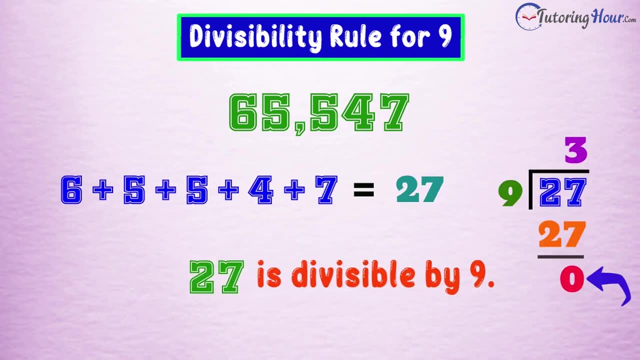 Add up all the digits and divide the number by 9.. Adding up the digits, we have 27,, and 27 is divisible by 9.. To simplify the process even further, we can repeat adding the digits until we end up with a 9.. 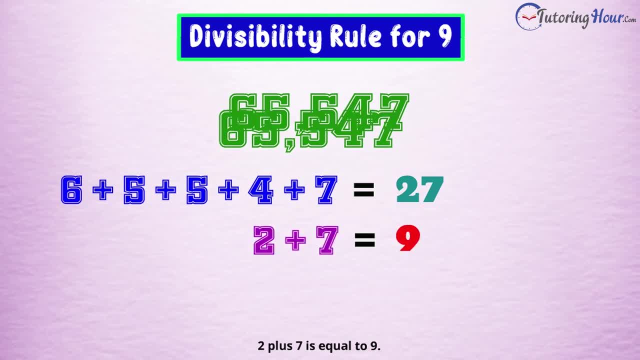 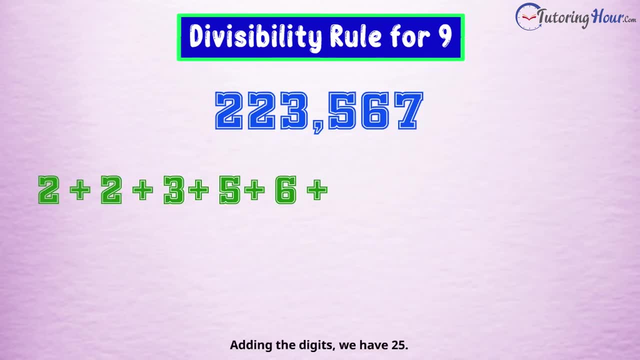 2 plus 7 is equal to 9,, hence the number is divisible by 9.. Let's try checking one more number Adding the digits we have 25.. We'll repeat the process and add up the digits 2 and 5.. 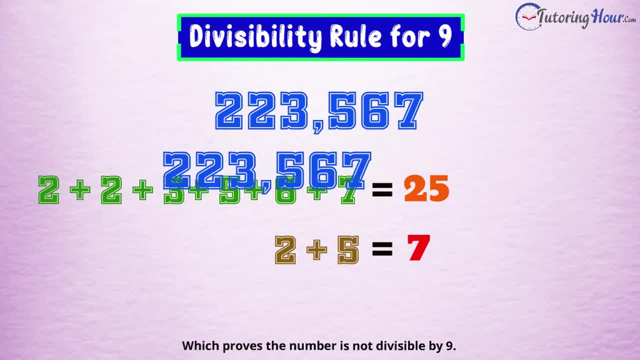 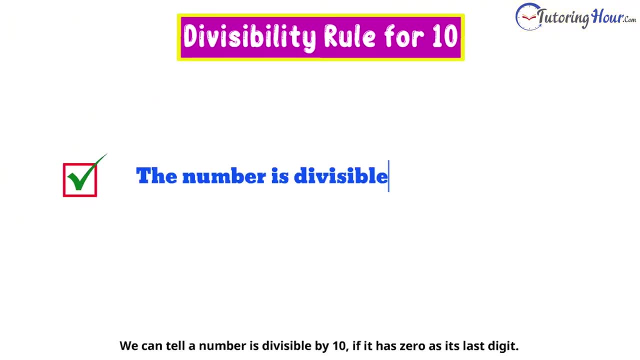 We'll end up with 7,, which proves the number is not divisible by 9.. Last but not the least, we can tell a number is divisible by 10 if it has 0 as its last digit. It is pretty obvious that this number is divisible by 10,. 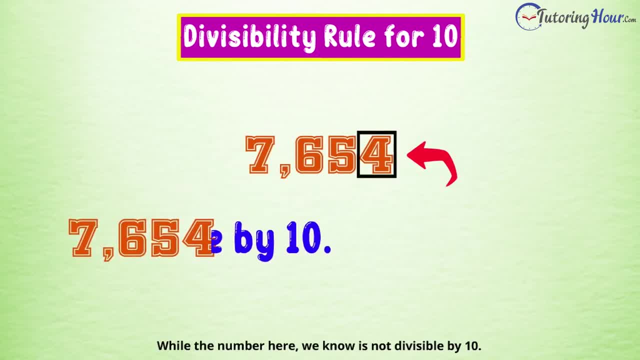 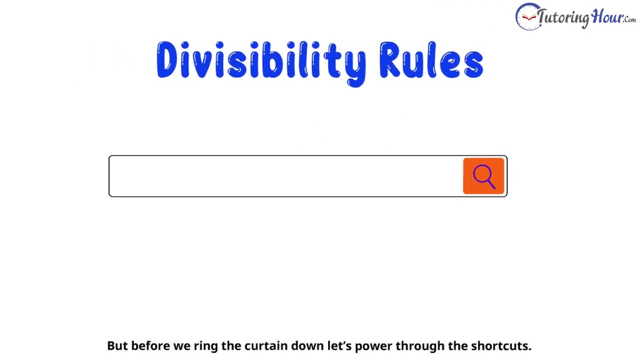 while the other here, we know, is not divisible by 10.. This brings us to the end of our video, But before we ring the curtain down, let's power through the shortcuts. Divisibility rule for 2.. The last digit is even. 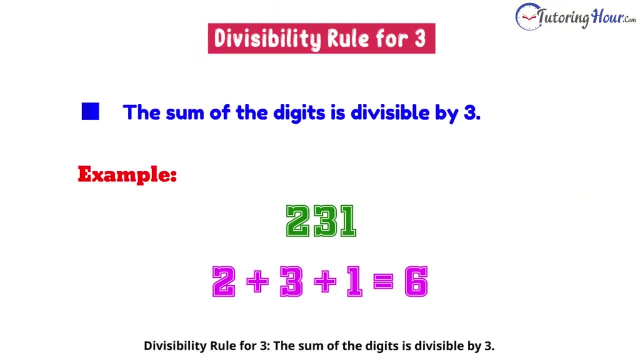 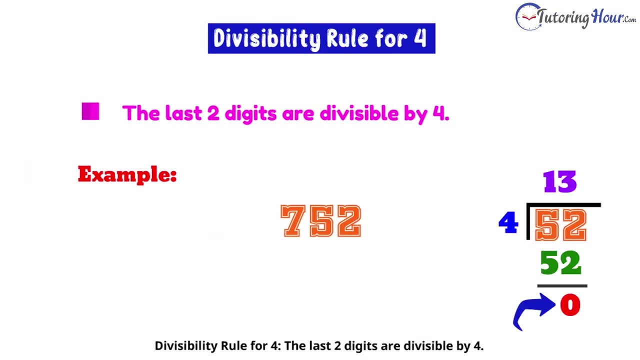 Divisibility rule for 3.. The sum of the digits is divisible by 3.. Divisibility rule for 4.. The last two digits are divisible by 4.. Divisibility rule for 5.. The last digit is 0 or 5.. 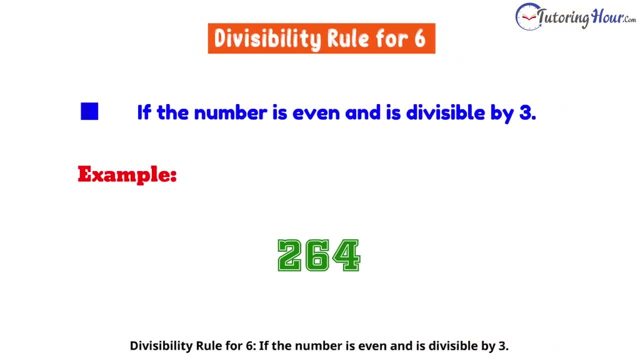 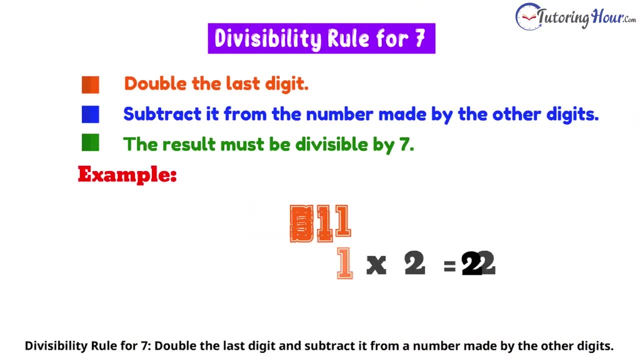 Divisibility rule for 6.. If the number is even and is divisible by 3.. Divisibility rule for 7.. Double the last digit and subtract it from a number made by the other digits. The result must be divisible by 7.. 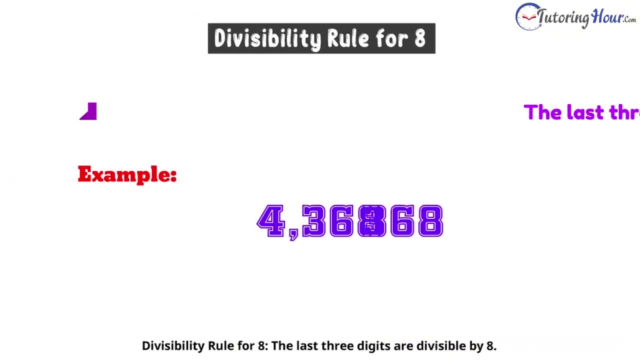 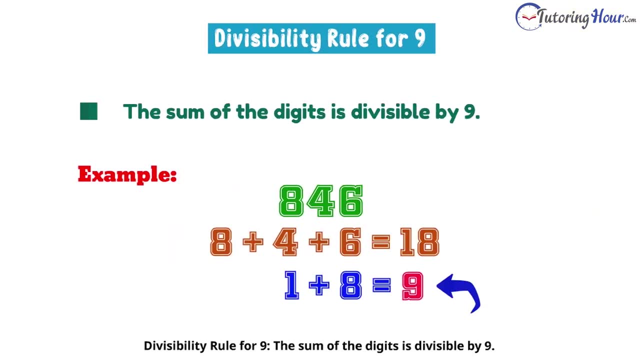 Divisibility rule for 8.. The last three digits are divisible by 8.. Divisibility rule for 9.. The sum of the digits is divisible by 9.. Divisibility rule for 10.. The number ends in 0..